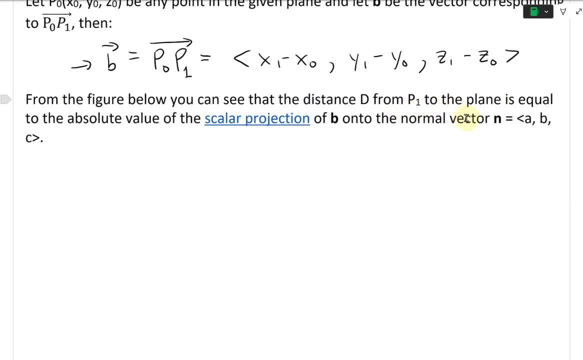 the distance d from P1 to the plane is equal to the absolute value of the scalar projection of B onto the normal vector. n equals to a, b, c. So let's make sense of all this And recall from my earlier video scalar projection. I put a link to that one there. 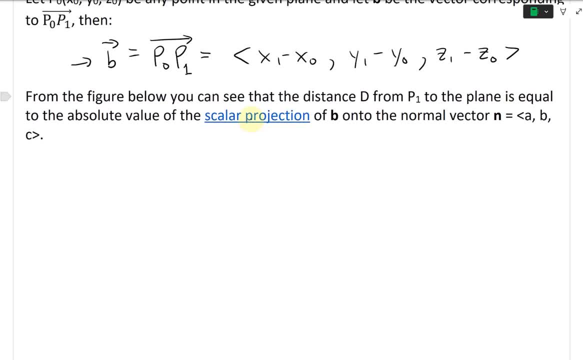 Yeah, so let's just make sense of all this and let's graph stuff out. So we'll have a plane like this. All right, a plane's going to be like this, All right. so the point P is a point P of P1 to the plane. 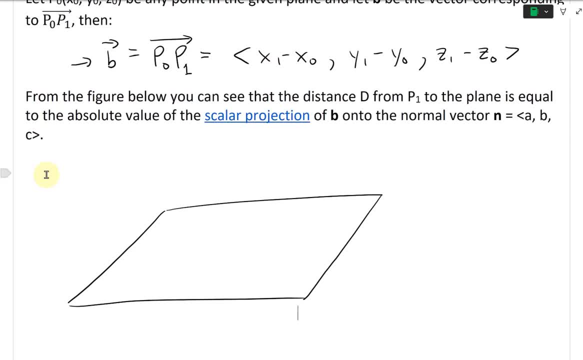 So the point P0 is on the plane. So let's say we had a point P0 here. This one is on the plane. So this is, P0 is on the plane, And let's say we had a point not on the plane or just any random point. 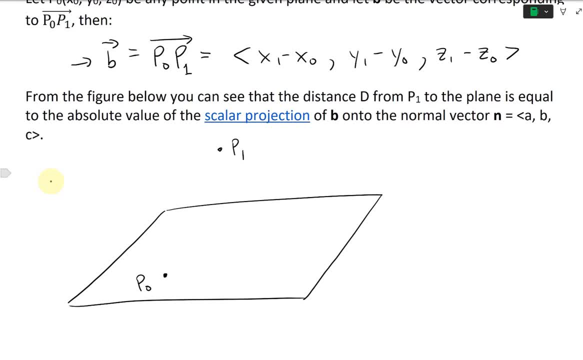 This is going to be our P1, like that. So that's P1.. And then the vector B is from P0 to P1.. So this vector right here, this is B, a vector like that, And now. so that's the plane. 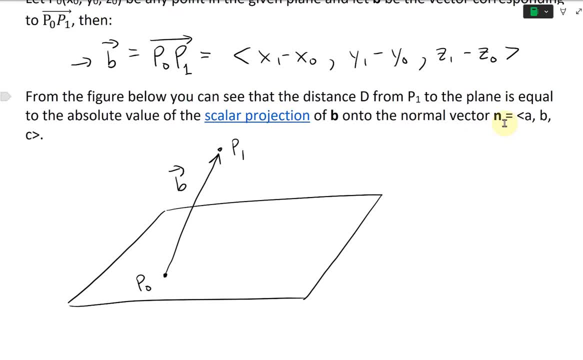 So now we have a normal vector here, n, And what we'll do is from the figure below we can see that the distance d, the distance d, is going to be well from. let's say, you had a point right across here. 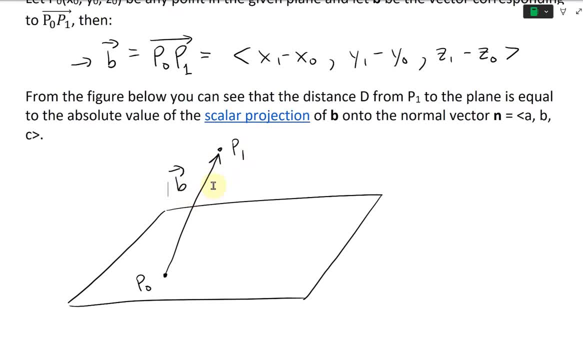 Or before we get to that. so let's say, look at this vector B. Now if we project this on onto the normal vector n, so the absolute value is going to be the distance. So in other words, if you project it all the way across to this point right here, 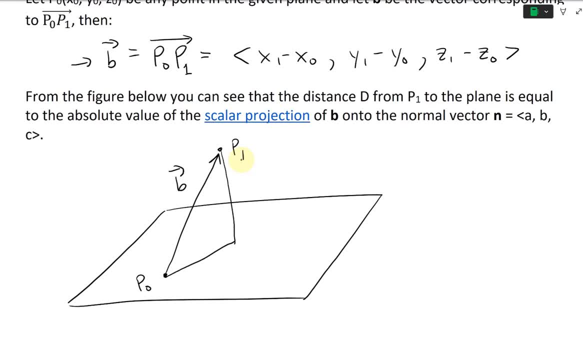 let's say, if you project it all the way across here to this, it's going to be a right angle. So we have this, we project this all the way on here, and then this angle is going to be- let's call this, theta. 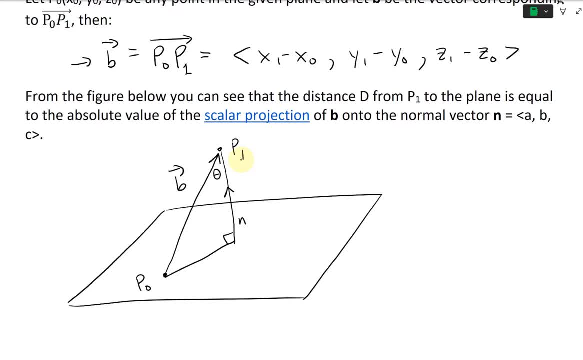 And then this from here to here is going to be n, So there's the normal vector, n. So then the distance right here is going to be from here to here is d. that's the distance from there to there, and it's just a scalar projection of this. 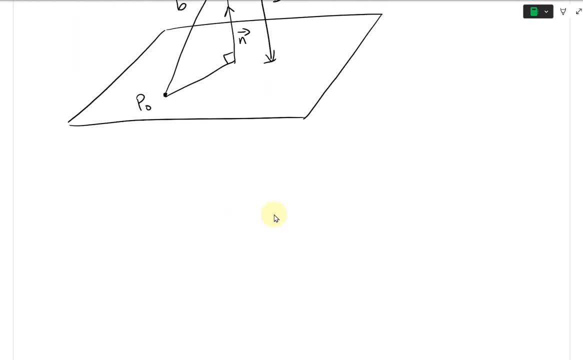 B onto it over there and first off recall. and we're doing the absolute value recall right here, if you look at just a basic trigonomic function. so we take the absolute value of cosine here cosine is going to be equal to adjacent over hypotenuse and Jason's D equals D over hypotenuse. is the absolute value of. 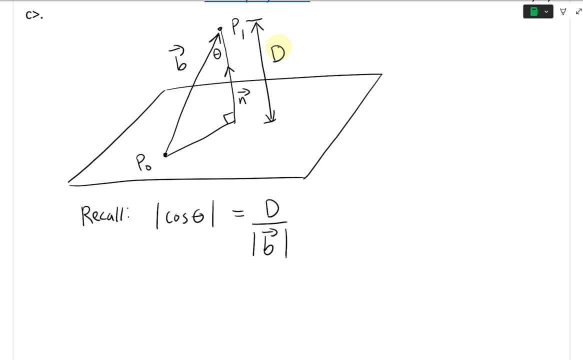 this distance B like that. yeah, so then this is so then a D is going to be equal to. so this over, it's going to be like this: the distance, the length of the, the hypotenuse B times by the absolute value of cosine. we're doing. 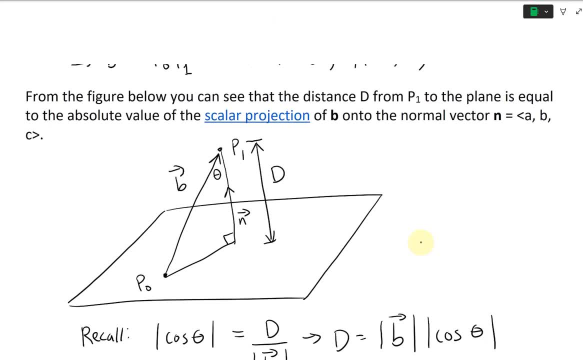 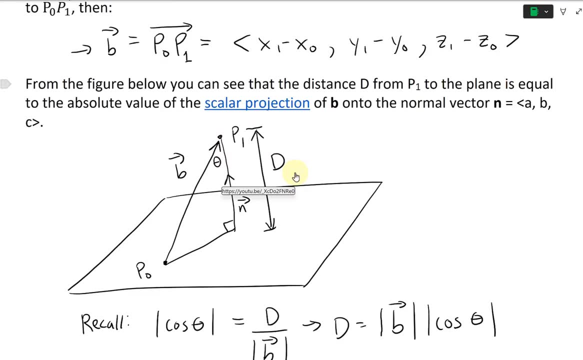 absolute values, just because we want the absolute values of all of these cosines and so on. yeah, since we're dealing with absolute values, I recall that this is from our other video, just a scalar projection of B. so this is the scalar and it's and the way you wrote it right, it is component. 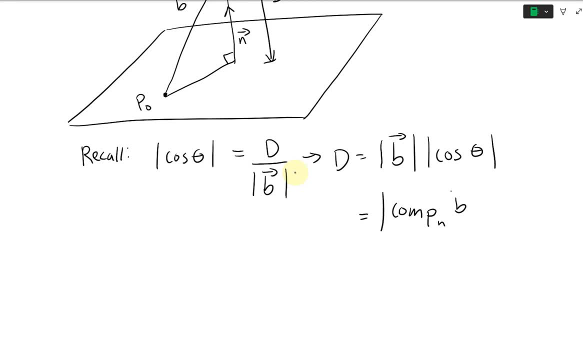 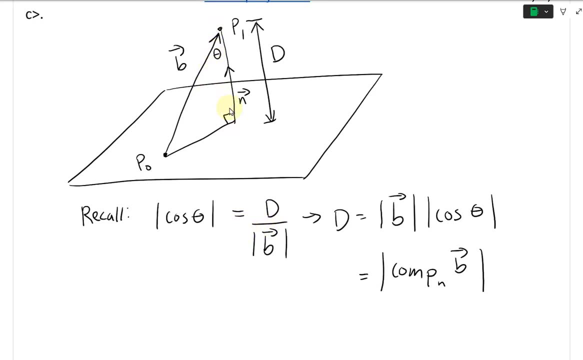 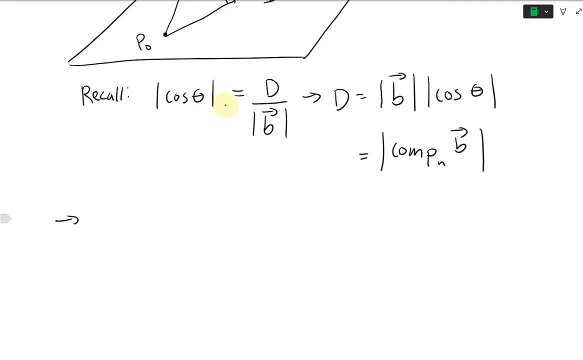 of of this is the component of B, on to enter the scalar projection. that's how you write it, but basically it's just this part right there. and also recall that this angle right here of these two vectors, B and N, that's just a dot product, so we can also apply the dot product. remember that cosine theta is. 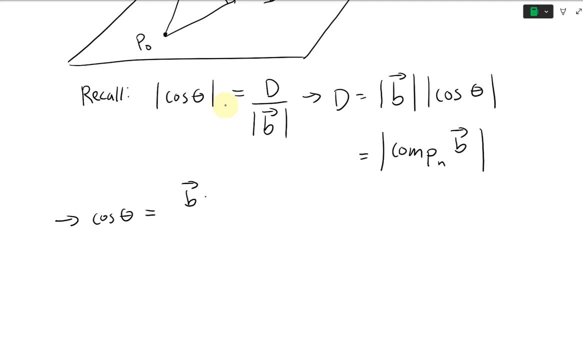 equal to B. I'll just write, recall this. and cosine theta is equal to the dot product of B, dot N, the two vectors with the angle between them, and then divided by the length B times by length N, like that. so then put this all together, what we end up getting is D equals to this right. 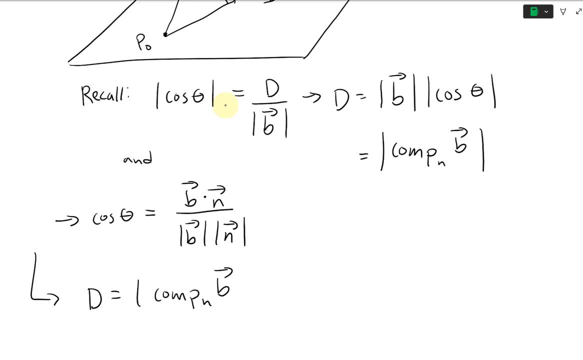 here, calm and the scalar projection. it's just the notation of how it's written. so this is the component of B on to N, believe that's how it's pronounced. all right, so we have this and then we're taking absolute value and then it's going to be the absolute value of that. it's going to be now. yeah, it's going to. 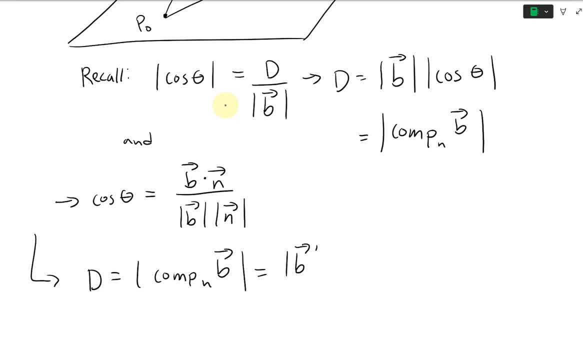 be this B, right there, the length B. then there's cosine. we put that inside. that's what this inside here. so it goes down here. it's going to be B, vector dot N. divide this by: there's a B on the bottom and like this: and there's the N, all right, 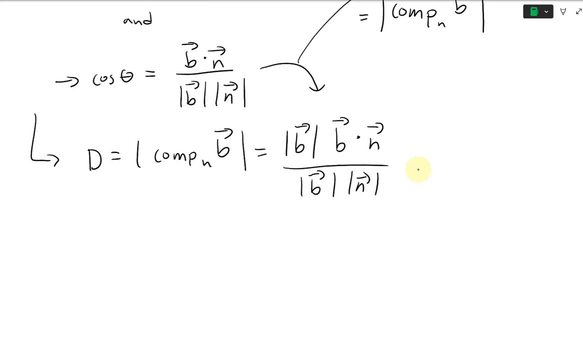 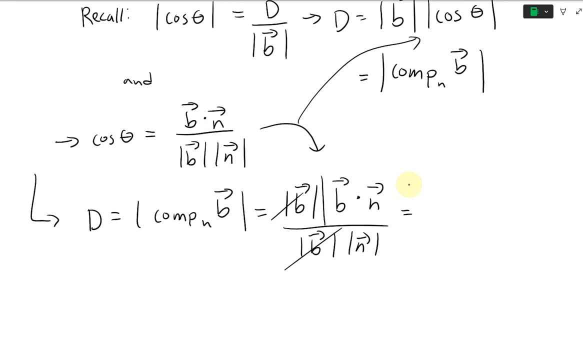 all right, yeah, computer just for us for a bit anyway. so we have this and this cancels, this cancels. so we're left with- and this is again we're doing- absolute value. so this whole thing is going to be absolute value. look at that in there. so 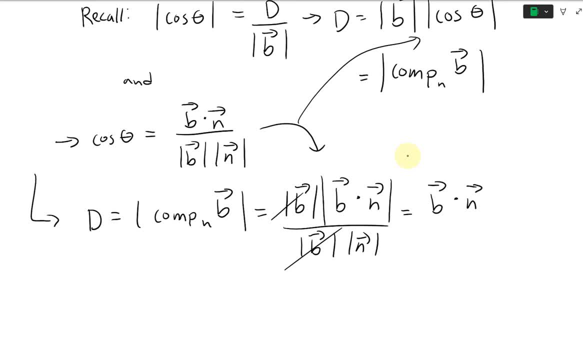 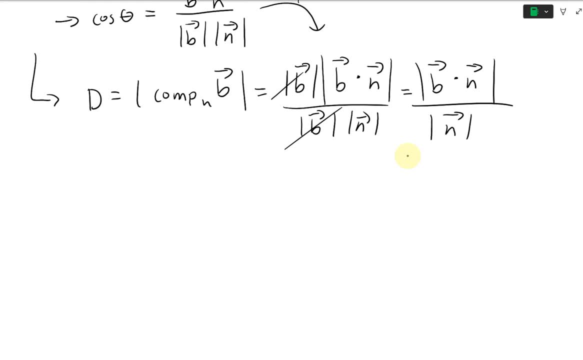 we get B dot, N dot, because we're doing absolute value of the distance and then divided by the length, N, like that. that's what we have. so, anyways, this equals to: yeah, this equals to the dot product. that's the value dot product. this is going to be, yeah, the B. 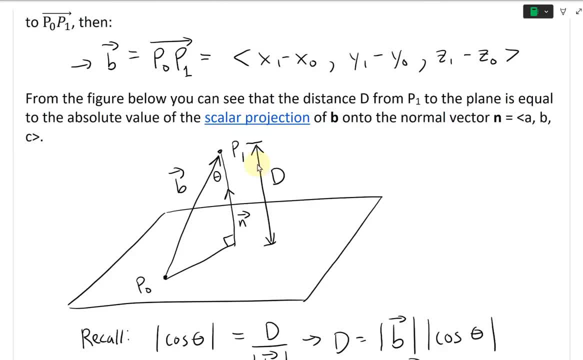 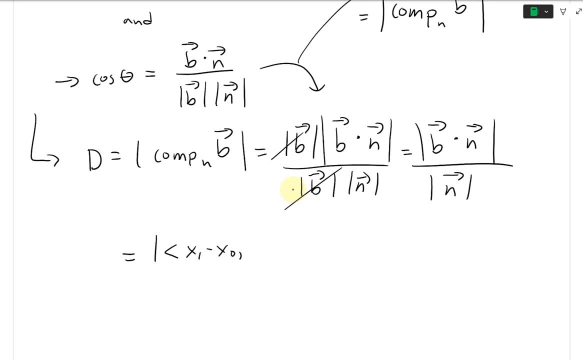 one right here is just X minus. yeah, it's just X 1 minus X naught, etc. this is right, all for completeness. so it's gonna be X 1 minus X naught. Y 1 minus Y naught, Z 1 minus Z naught. 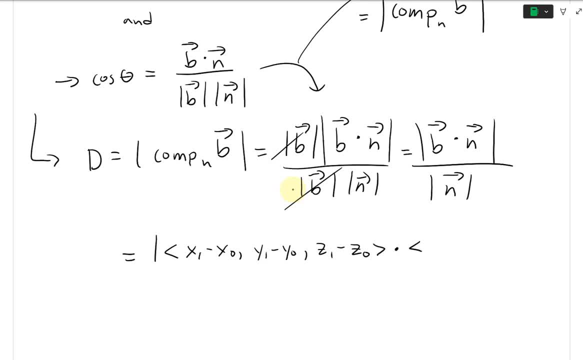 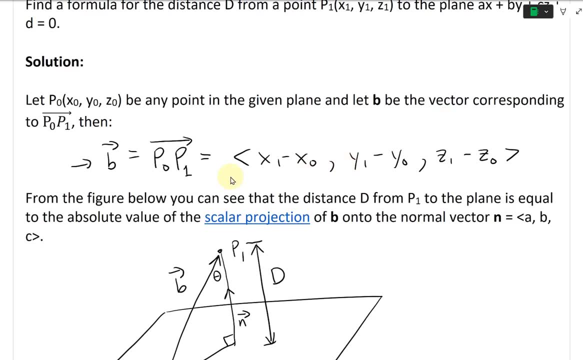 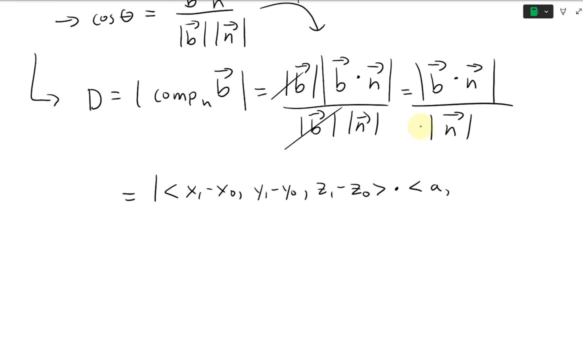 then dot, then the vector, and it's gonna be ABC. yeah, this, and it's just gonna be the ABC. yeah, as per here. so a normal vectors ABC like that. all right, it's gonna be a, B, C and then absolute value divided by the end. the bottom is going. 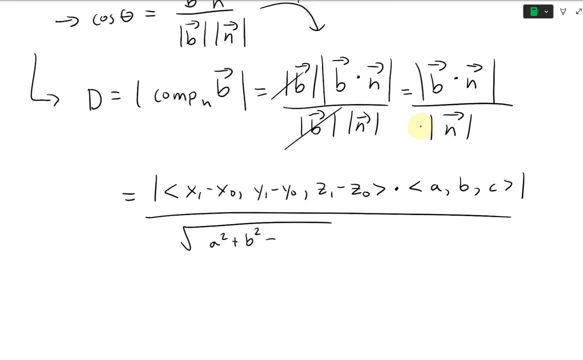 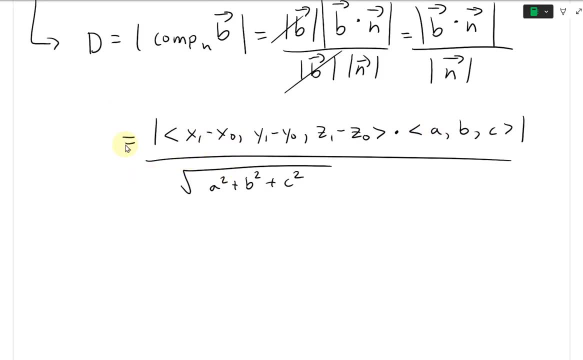 to be the length. it's going to be a squared plus B squared plus C squared of the normal vector M. yeah, so then now. so then what we ends up getting is multiply the a inside, keep going, so we're gonna get a. put the triangle bracket in front, so 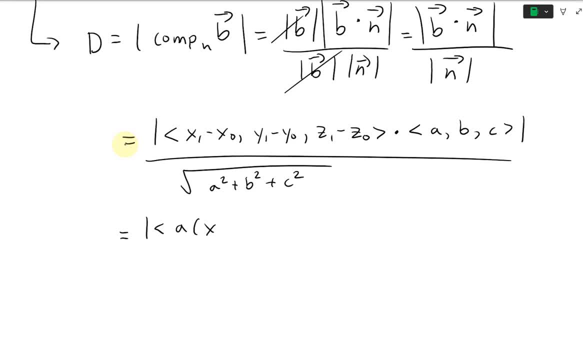 we're gonna get a X. actually we're not doing the triangle bracket because we're doing a dot product. so the dot product is is a scalar. so then it's going to be a X 1 minus X naught plus B. X 1 minus X naught plus B. X 1 minus X naught plus B. 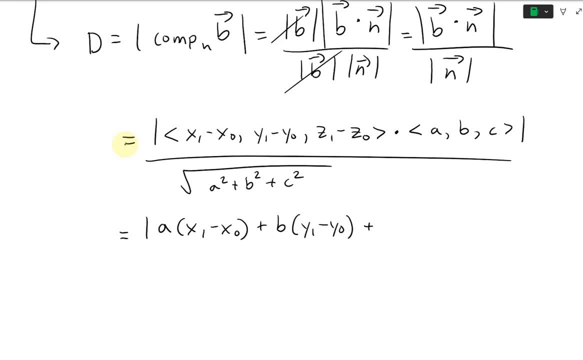 Y, 1 minus Y, naught plus C, Z, 1 minus Z naught, like that absolute value. and then divided by and again, it's frozen. so divide this by scalar: a squared plus B squared, and plus C squared like that. so that's what we have. and then what's next? 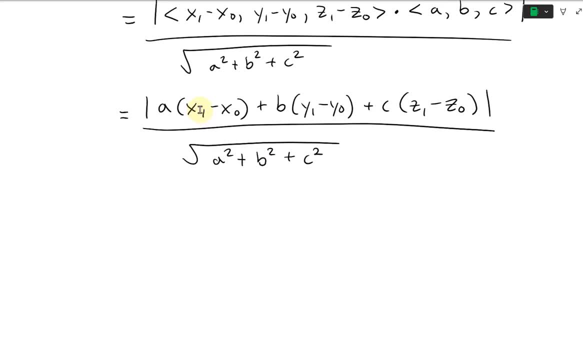 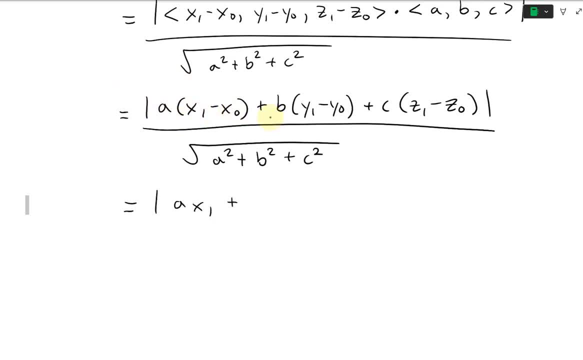 multiply all these together and the other ones are separately: plus B, Y 1, plus C, Z, 1, and then we're gonna have minus. this is going to be minus, and then put a bracket- a, X, not, then the next one here is gonna be minus, and there's a B plus B. 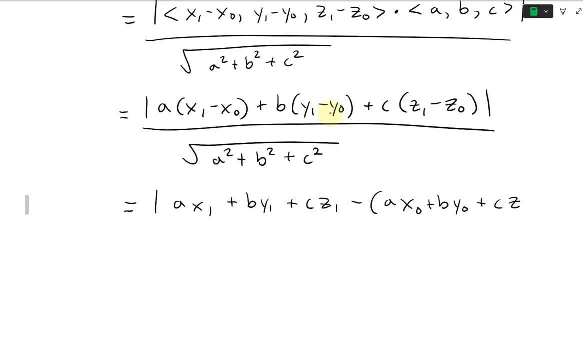 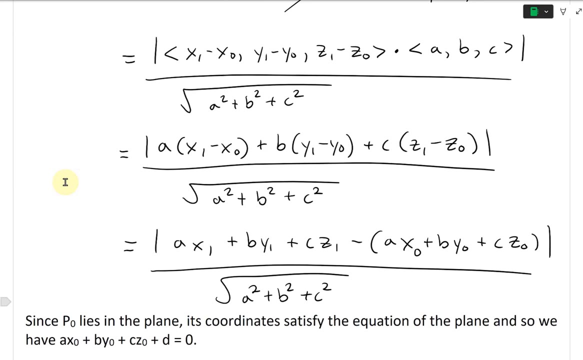 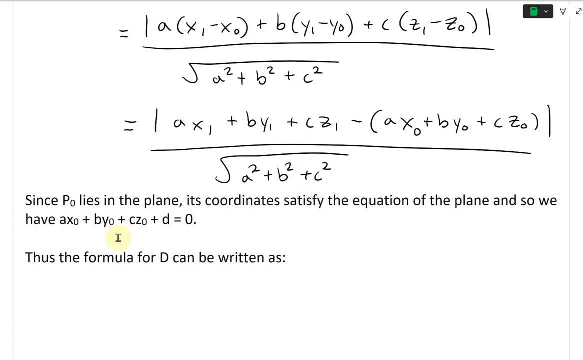 why not? so we took the negatives out. plus C is a, not like that. and again, divided by a, squared plus B, squared plus C, squared like that. alright, so now that we have all this. so since P naught lies in the plane, its coordinate satisfies the equation of the plane. so we have a X naught plus B, Y naught plus C, Z naught plus D, E. 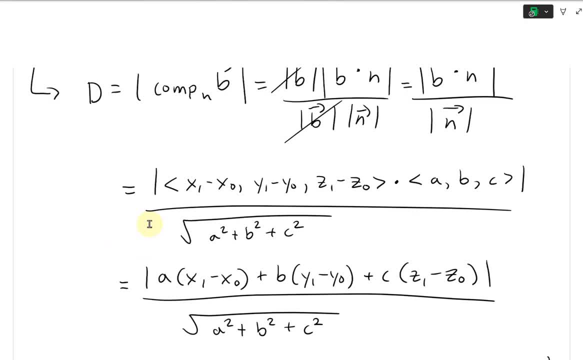 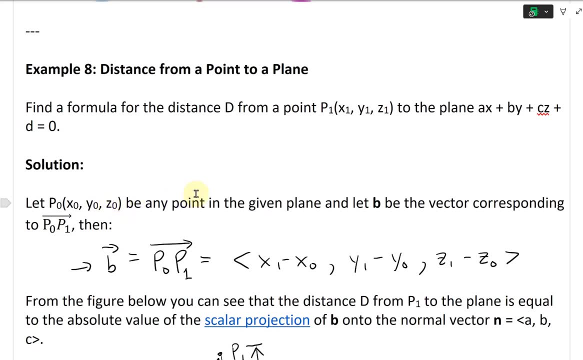 Ymb equals to zero. Yeah, now we can see that above here. So we again, we were. we let p- not with coordinates x, not y, y not z- not be any point on the given plane right here. So if you plug in, 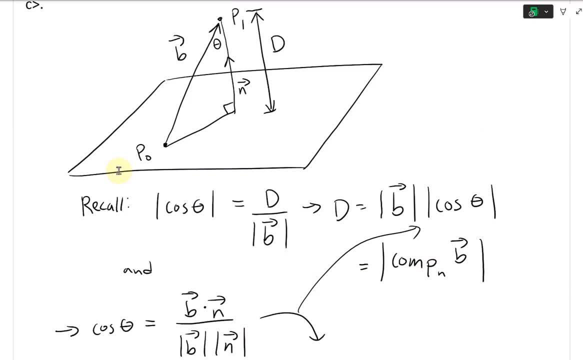 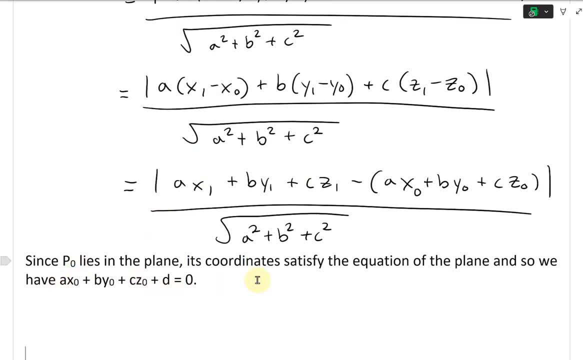 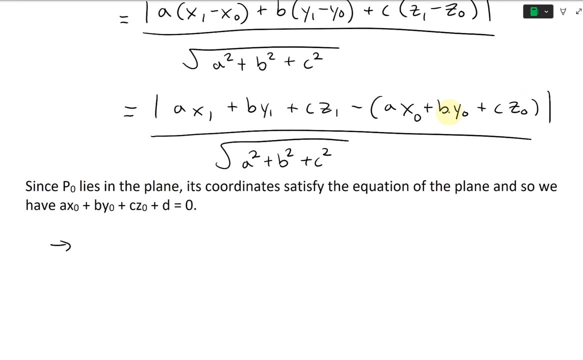 these x, not y, not z, not. then then yeah, that just equals to zero plus equals zero. So in other words, this part right here, let's move this like this, make some room. So then what we'll get is: if we write it like that, we'll get, if you make this whole thing over to the other side, we're